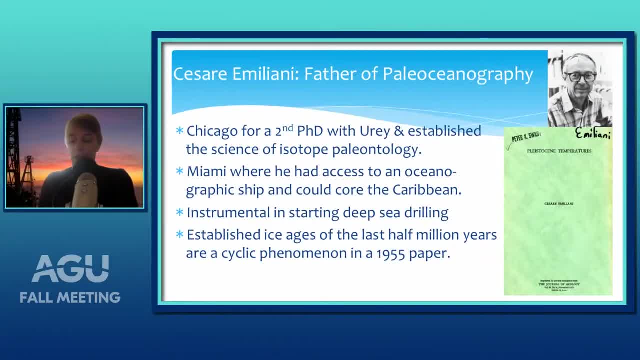 foraminifera's growth and he showed for the first time that ice ages are a cyclic phenomenon, and this gave strong support to the Milankovitch hypothesis and revolutionized ideas about the history of the planet, oceans and climate. His paper from 1955 still receives an average of about 20 citations per year, more than 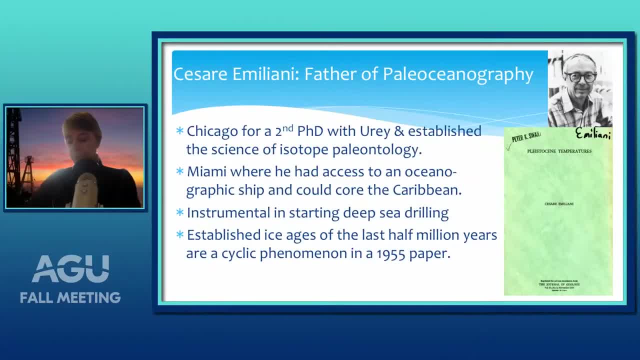 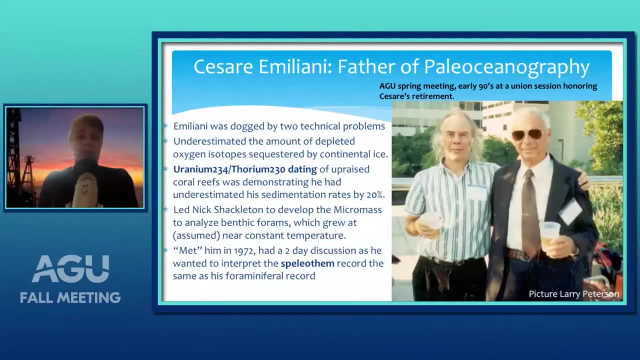 50 years after its publication. There were two technical problems that dogged Emiliani. One is that he underestimated the amount of oxygen isotopes sequestered in continental ice, and this led others to develop the field to solve these issues. For example, it led Nick Shackleton to develop the micromass on mass spectrometers to analyze. 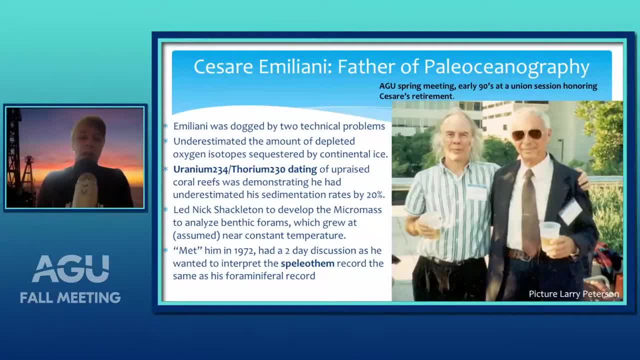 benthic foraminifera, which grew at what we assumed at the time to be a near-constant temperature. He also underestimated his sedimentation rate by about 20%, and it took dating from other types of geological reservoirs to demonstrate this. Usually also at this point, speakers. 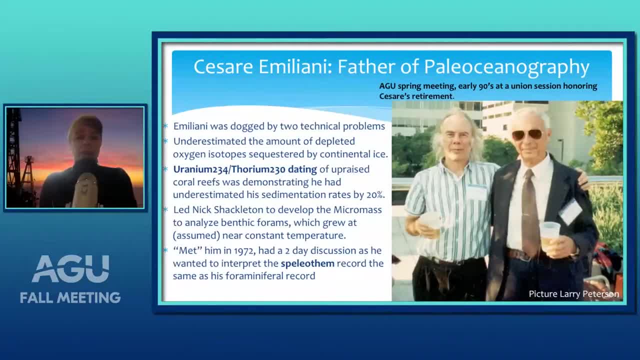 talk about how they met César. I'm not going to go into too much detail on that. I'm just going to give you a brief overview of Emiliani and their interactions. So I did meet him in 1972. I was six months old and there was an intense two-day discussion. 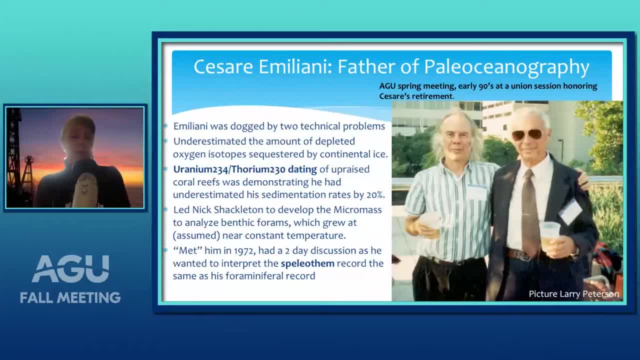 where he wanted to interpret my father's speleothem records the same way he interpreted his foraminifera records. So that is my connection. Elizabeth Sykes, this year's Emiliani lecturer, began her career with the idea of studying geological isotopes. 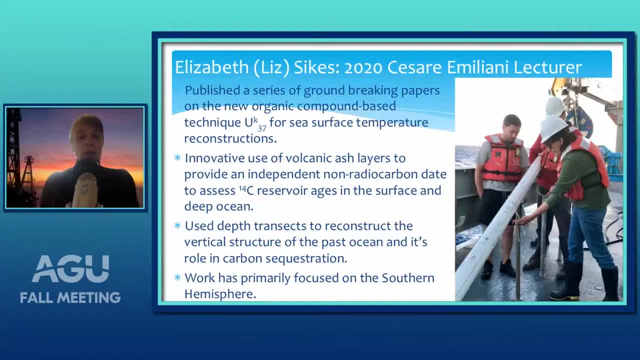 She was a professor at the University of New York and she was a professor at the University of New York. She was a professor at the University of New York and she was a professor at the University of New York, and she was a professor at the University of New York. 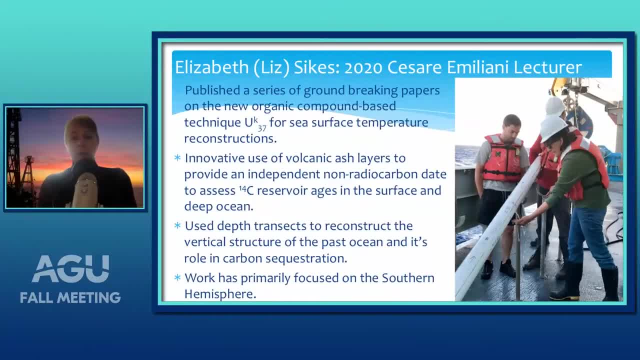 They were working in organic compound techniques. She published a series of groundbreaking papers for generating sea surface temperature reconstructions using alkanones and these papers today are highly cited. And she used this work and has continued to use this work in the southern hemisphere to 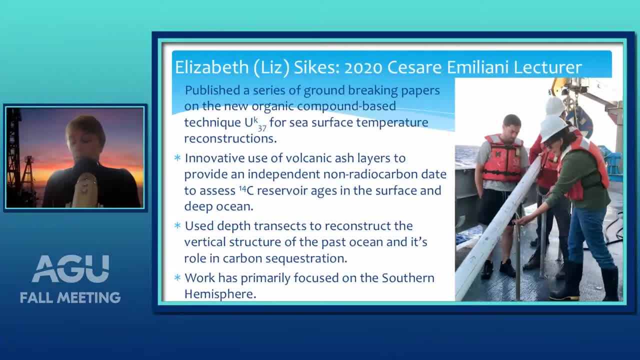 provide critical information about movements of ocean fronts, of the winds- southerly, the southern westerly winds, and the Pacific Ocean, the Southern Ocean. I first encountered Liz when she was doing her work off New Zealand: innovative work using volcanic ash layers to provide independent non-radiocarbon dates to assess surface ocean and deep ocean reservoir ages. 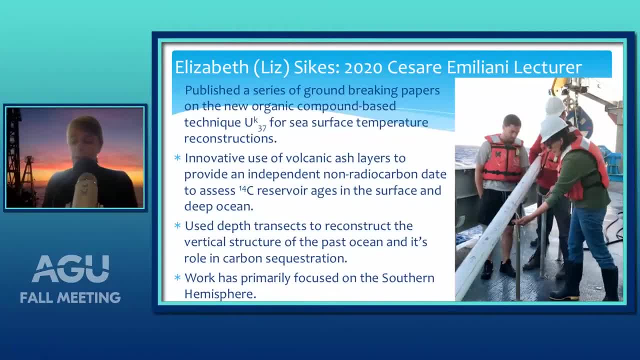 Her work here contributed to our understanding of how the deep ocean sequestered the missing CO2 during glacial intervals. These are the cold intervals of the Milankovitch cycles that Emiliani helped support. Much of her work in the Southern has focused on the Southern Hemisphere and the Southern Ocean. 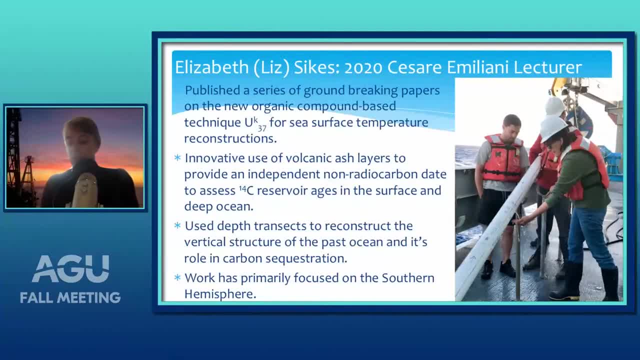 She's used depth transects to reconstruct vertical structures of the past ocean and demonstrate its role in carbon sequestration, to show how the Southern Hemisphere and the Pacific Ocean are interrelated. The Southern Hemisphere winds led thermohaline circulation changes to drive CO2 out of intermediate water depths. 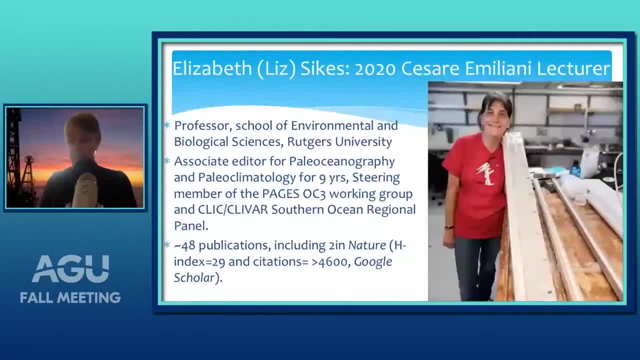 Throughout her career, Liz has generously invested her time to provide intellectual leadership and to serve the community. She is currently a professor at the School of Environmental and Biological Sciences at Rutgers University. She's been an associate editor of Paleoceanography and Paleoclimatology for nine years. 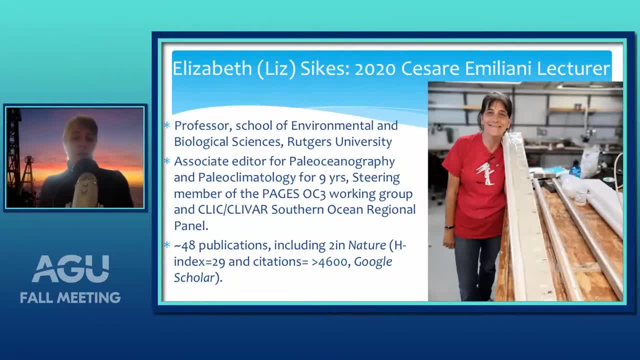 with the PAGES OC3 Working Group and the CLIVAS Southern Ocean Regional Panel. Liz embodies the scientific spirit of César Emiliani in that much of her efforts have focused on development and testing of paleoceanographic methods, And I welcome Liz Sykes as this year's Emiliani Lecturer. 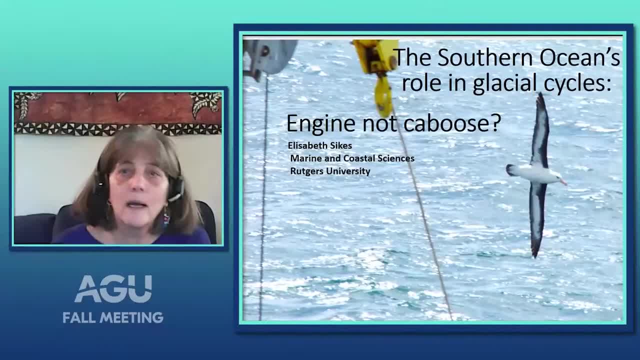 Good morning. My name is Liz Sykes and I'm very pleased to be here giving you the Emiliani Lecture For 2020,. I have been working in the Southern Ocean for most of my professional life. Why, I like to say that's because that is where the Southern Ocean, the Southern Ocean is where the ocean exhales. 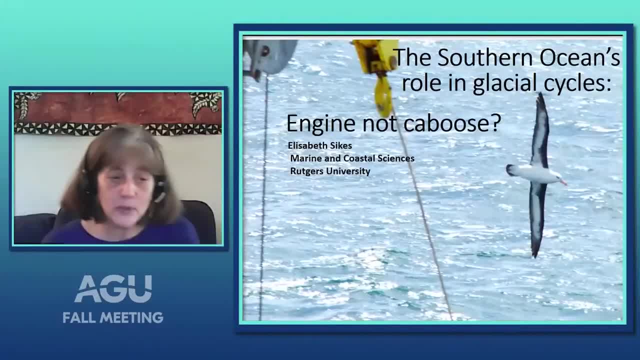 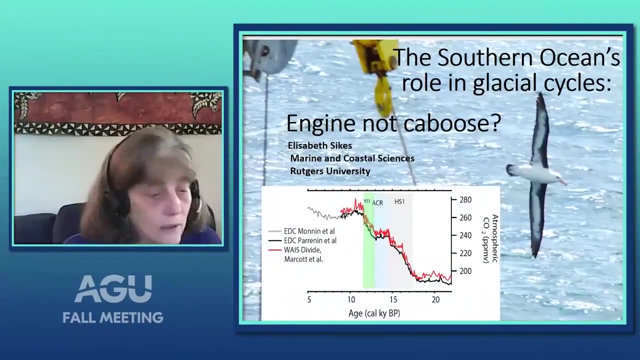 We've known. we know that the deep ocean holds 50 times more CO2 than the atmosphere today And in glacial times we know that the ocean held even more CO2 than today, And what I'm showing here is one of the most important paleoclimatic records from the last 50 years. 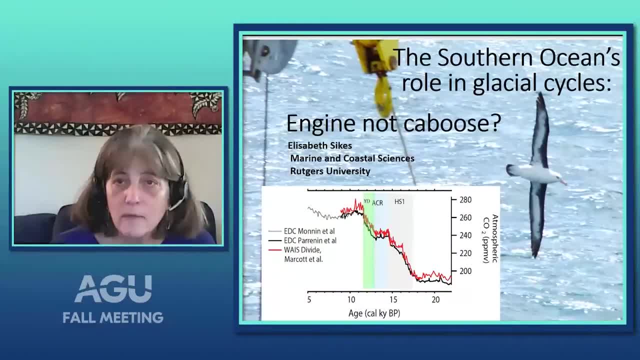 This is the record of CO2 taken from gas- atmospheric gas- in ice cores, And what it shows us is that in the last glacial maximum, about 20,000 years ago here, that the CO2 in the atmosphere was one third less than today. 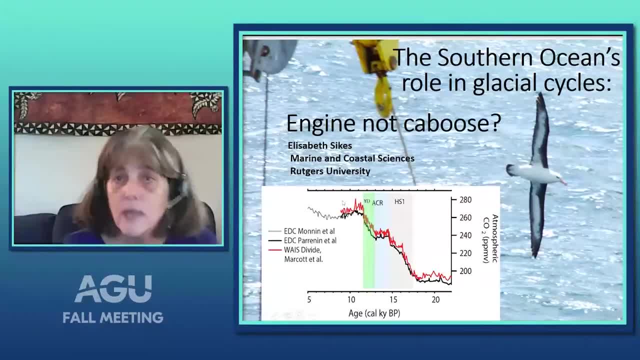 And over the course of less than 10,000 years, the atmosphere CO2 content increased by a third. The rapidity of that change is one of the most important diagnostics for us to understand that it had to come out of the deep ocean. 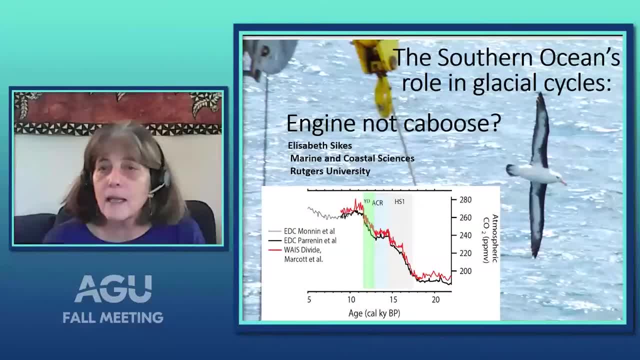 That's the only other reservoir of CO2 on the planet that could deliver that much CO2 to the atmosphere in that much time. So although I think it's very well understood that probably the basic forcing for climate change is insulation- The amount of solar energy coming into the planet- and that CO2 is an amplifier- 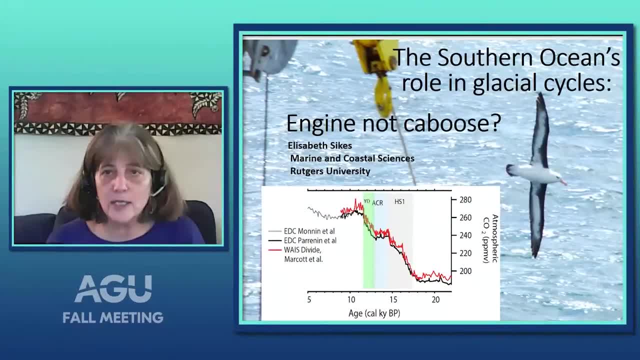 So to understand the Earth's climate changes, we need to look at both. So another thing that's important about this record is not just So. the CO2 is an amplifier on the solar radiation And one of the important pieces in that is looking at the details of this record. 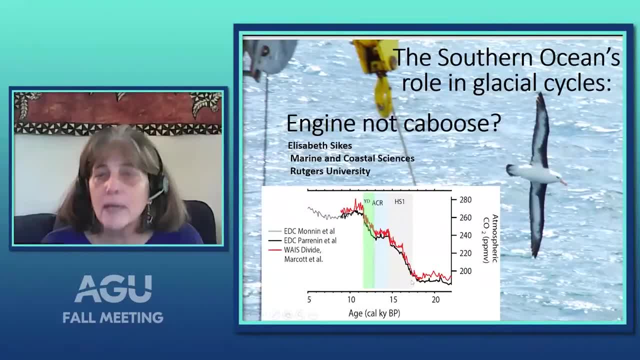 So not only was this CO2 change very rapid, but it came in steps, And so, with the first rise being during Heinrich Stadion I, a pause during the Antarctic Cold Reversal and another rise in the Younger Dryas. 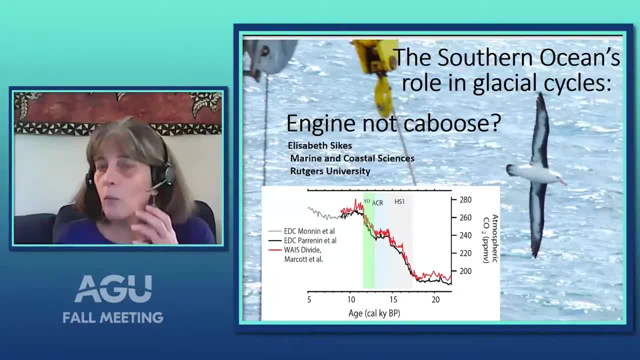 And so one of the questions is not what the basic mechanisms of how the planet came out of the last ice age, but what are the details of it, What are the drivers of that change, And so one of which I think most would agree, as I said,